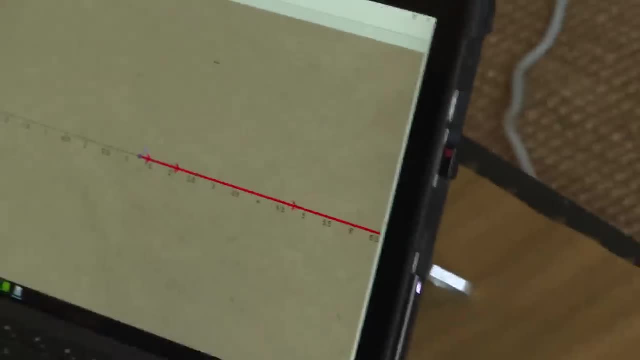 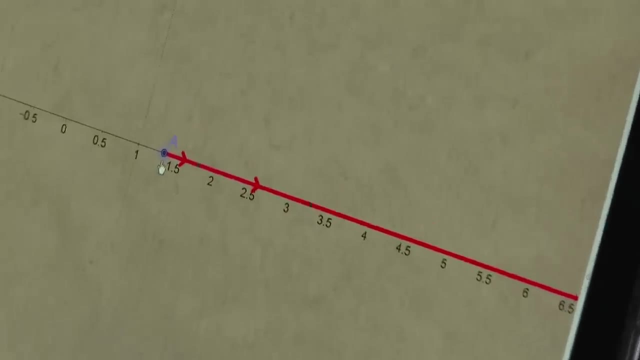 not, and it's best to see this on a diagram. So have a look at my screen here. You picked the number seven, which is kind of off my screen here, but these red arrows I'm moving them around. this is not the greatest diagram. let me get this clear. to start with, It's just a line. 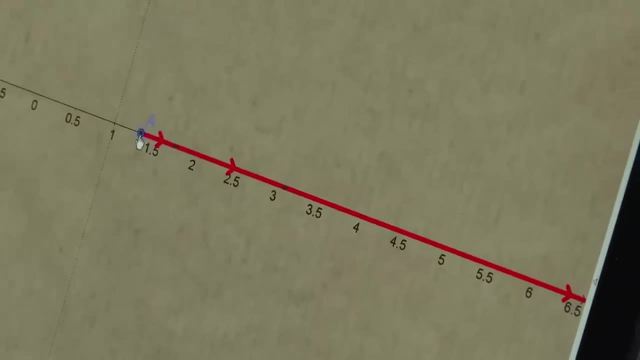 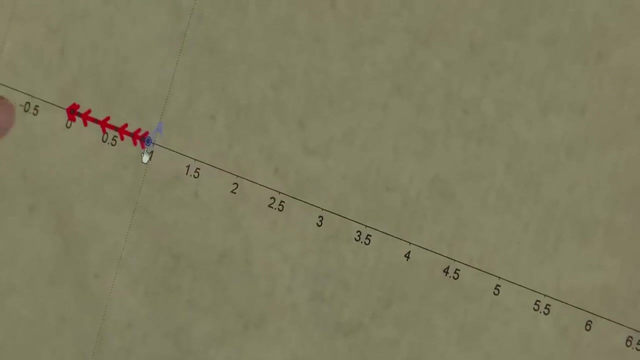 but the arrows are heading that way because when I square this number, I'm moving around, they go that way And they never come back, much like your seven did. But if I go less than this number one, they don't go that way anymore. they go that way, In fact, they head towards zero and they're stable. 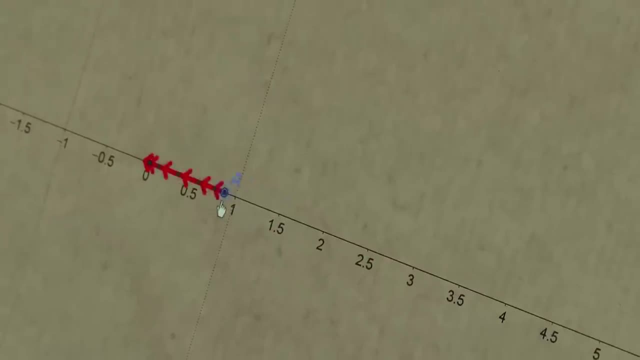 there. So for the sake of moving it around, it's kind of nice to see the difference. it's a really sharp line and it completely changes behaviour. but that way they're unstable. that way they're stable, Stable, unstable, stable, unstable, stable, stable, unstable. you get the idea. 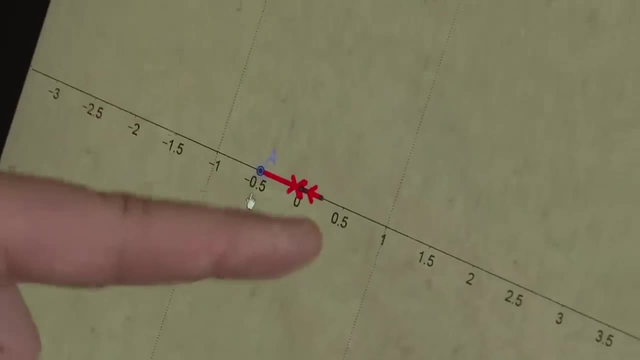 In fact, if you go negative, they're still stable. they head positive because when you square a number that's negative, they get positive, Still, head towards zero until you hit minus one, and then unstable, stable, stable, unstable stable. Now, despite all my commentary, it's not that exciting. 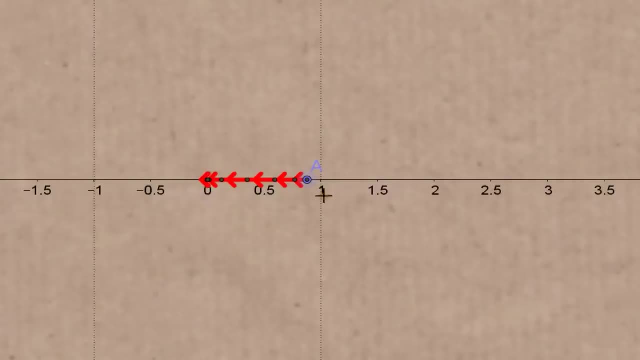 yet, and if you know anything about the theory of iterations and the consequences of them, or if you've watched any other video about the Mandelbrot set, you know that we're not just talking about real numbers, ie the numbers on the line I've just been showing. 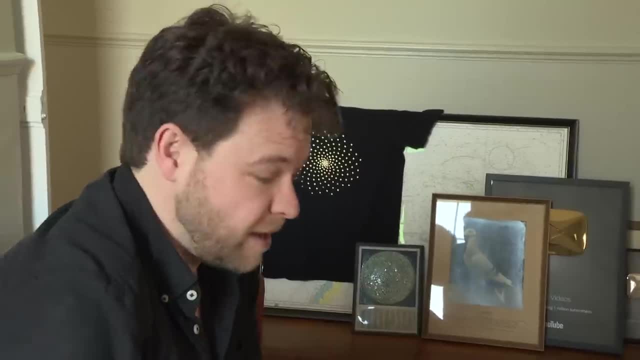 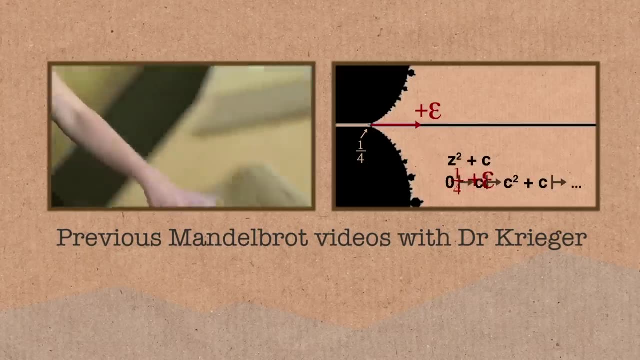 you. we're talking about numbers in two dimensions, so complex numbers, And I'm not going to give you an introduction to complex numbers here because I don't think you need to hear it and there are other places you can get them. Holly on the Numberphile channel has done excellent videos. 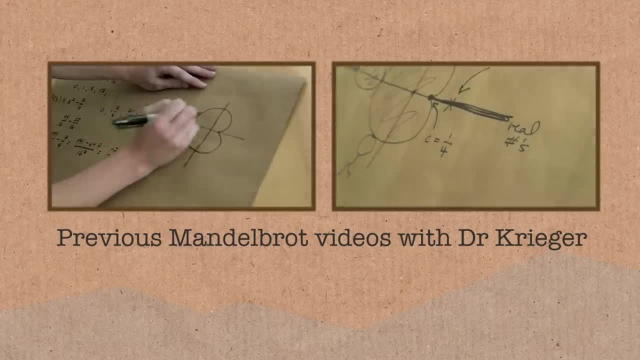 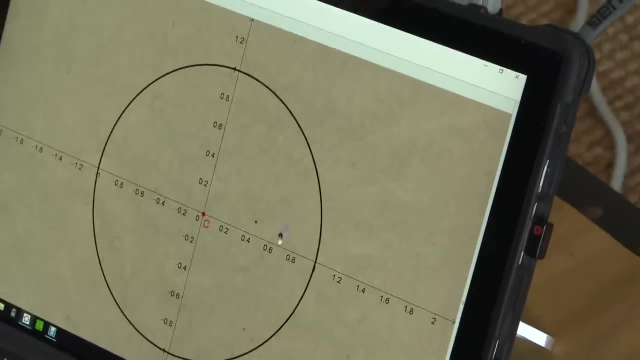 about how this happens, but I want to show you the same comments that she's made on brown paper. I'd like to show you moving. Here's my two-dimensional number line. Here is the number that you get to pick randomly. We can still do it in one dimension just by sliding along here. 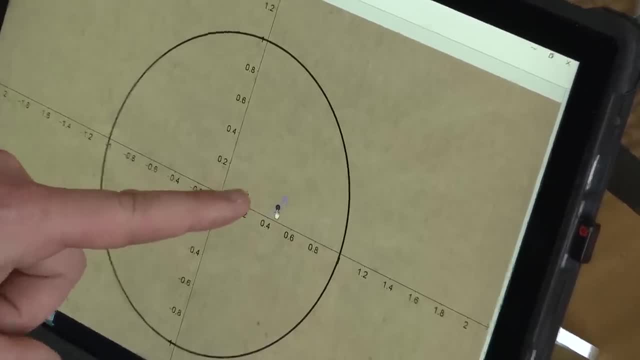 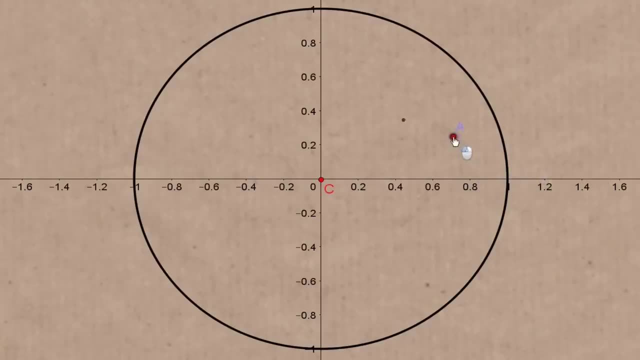 and the other dot that's moving around. this tiny one is the square of the other dot, So one squared is about one bigger than one. it heads off that way. lower than one, it goes that way. but I can move off the line now and it has a weirdly circular flavour to it which I kind of like. It's like chasing the number around. 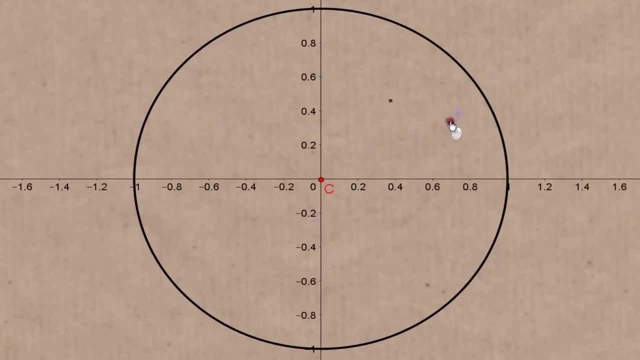 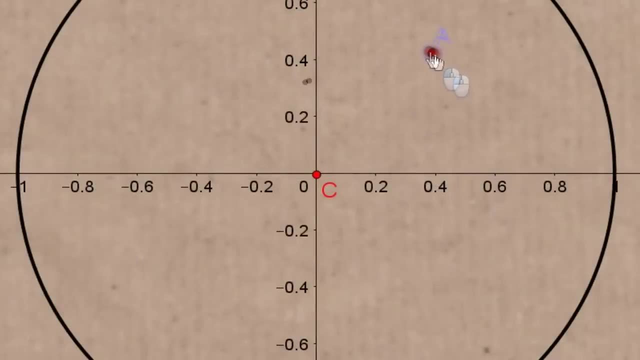 It moves quicker than you expect, and that's already quite pleasing if you're a nerd like me. but what I'm really interested in is the iteration. If you keep doing the instructions, square it, square it, square it. we saw what happened on the real line In two dimensions. 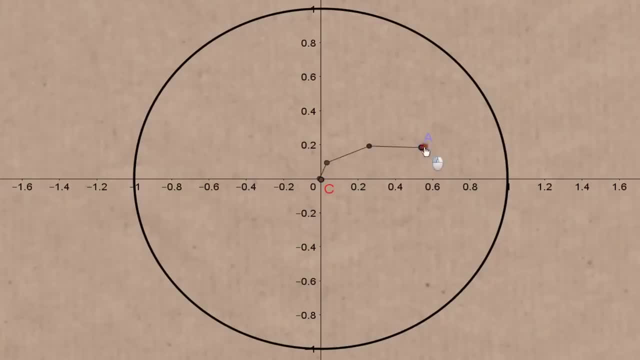 it looks different. So it looks like this. So this line indicates if you start there, it goes to there when you square it, and then to there and to there, And so if I move this around, the picture is kind of pleasing, kind of wobbles around, but it's always heading towards the centre, which I'll say is: 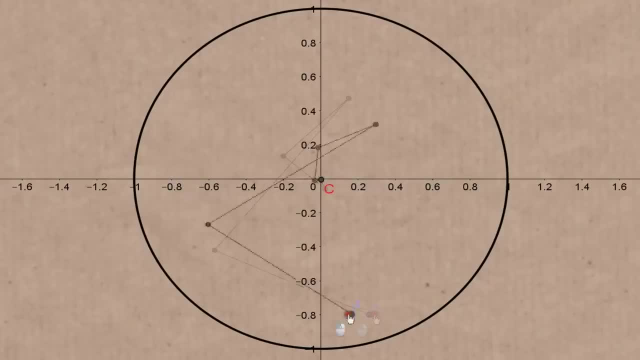 stable And there's a reason there's a circle on the screen, because any time I'm inside this circle it looks like it's stable, even if it's kind of pretty as it moves. But if I go near the edge of the circle it's less obviously stable. It takes a lot longer to get to the centre and then if I go, 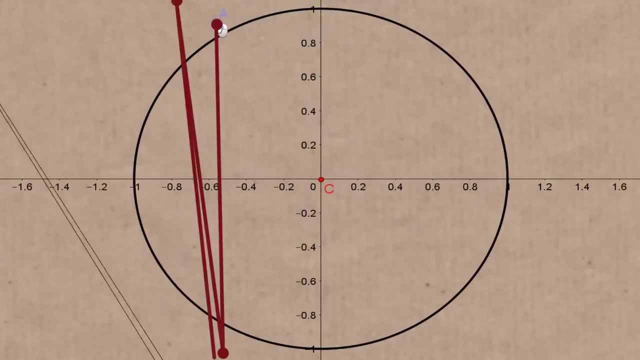 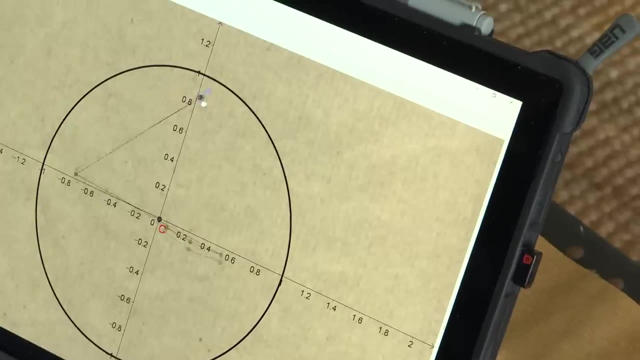 outside the circle: unstable, Stable, unstable, stable, stable, unstable stable. This is a really nice demonstration of why complex numbers work. A lot of people think that complex numbers are helpful in that, instead of your entire image of what's happening. 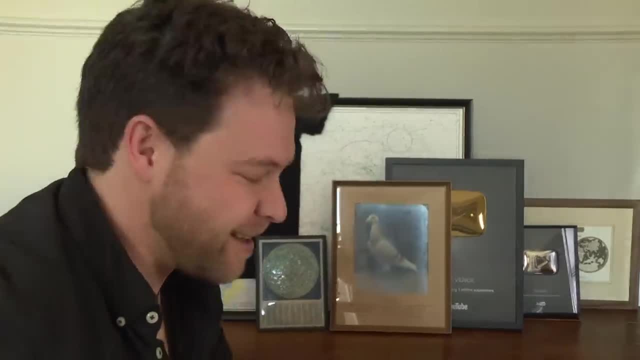 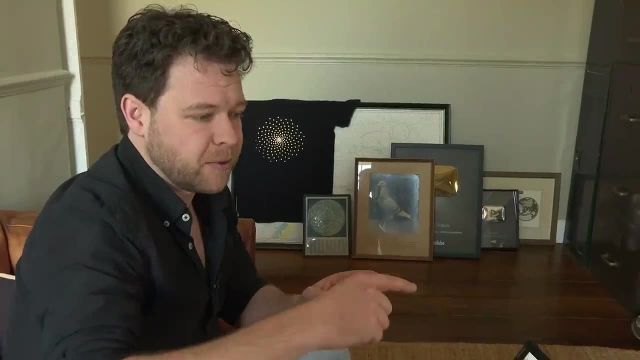 being on a line. you've got a picture, But it gets better, right, Instead of just squaring it. what would happen if you did: square it, add something. square it, add something, square, it, add something. Now we could go back to the real line and see it happening on just one dimension, but 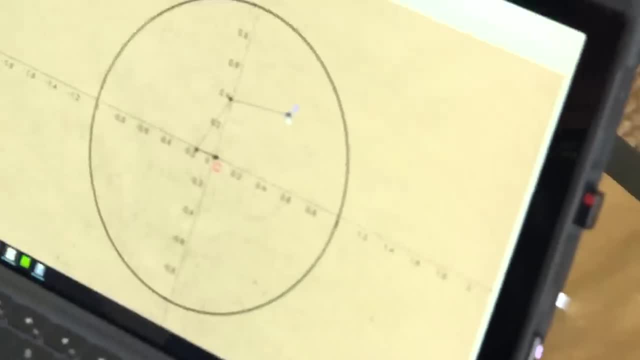 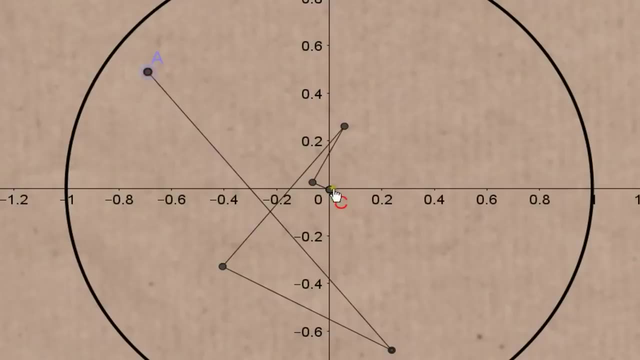 I feel like we should just go straight into two dimensions. This is just the square: square, square, square. This letter c is indicating a number I could add every time, So let me just slide it away from zero. At the moment it's not adding anything, but if I add this number, 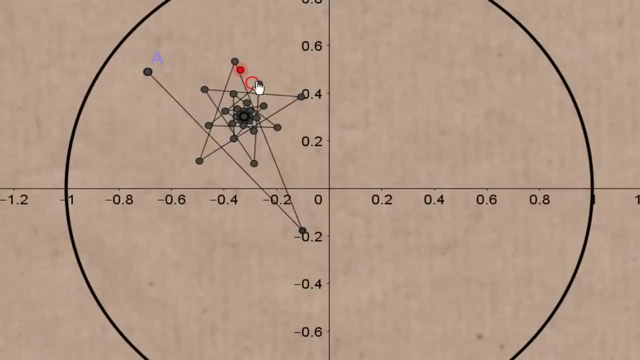 this red number, which is a complex number, it's two-dimensional. you can see, something very different has happened. If I start with this number and I keep squaring it and adding that number- square, it add that number. square- it add that number. square, it add that number. 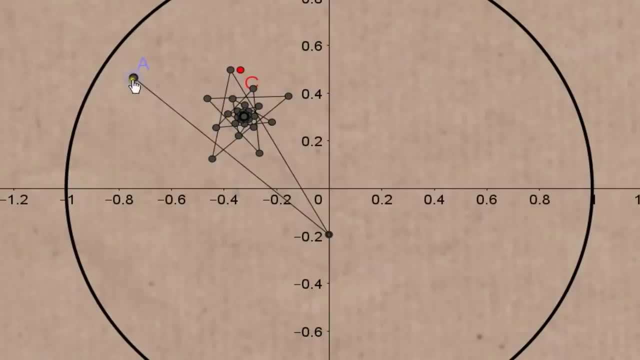 this is the path it goes, And it makes a lovely star shape. What's interesting, though, is not just the star shape, although I kind of like it. it's the stability. So all around here it's stable, and it always gives you the same sort of stability, like the starry stability, even if it's expanding. 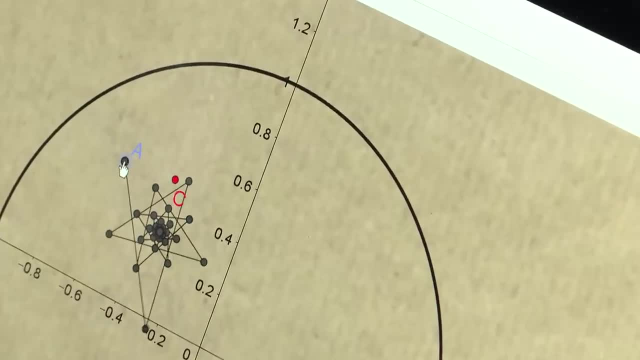 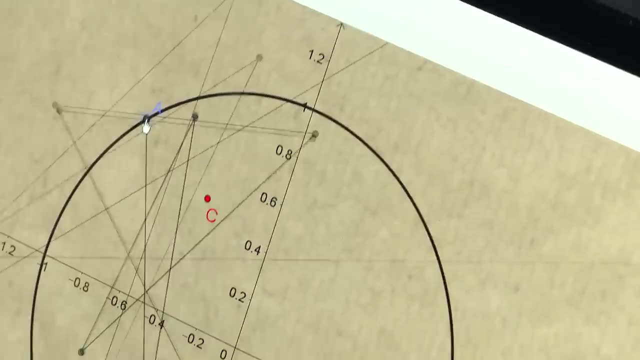 or shrinking. But you kind of get the feeling that sometime it's going to blow up, and it's not obvious where, because if I go near the circle you think it's going to blow up. it's going to blow, but it doesn't. So there was a moment there, so outside the circle still stable. 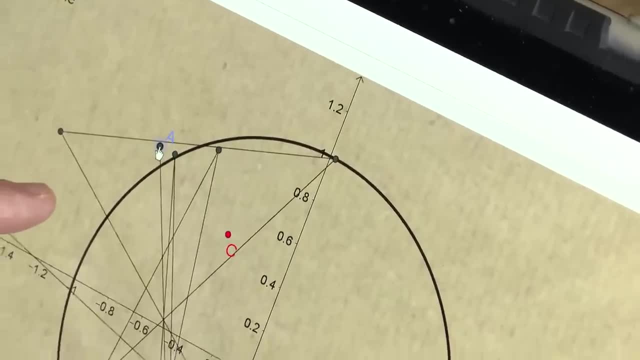 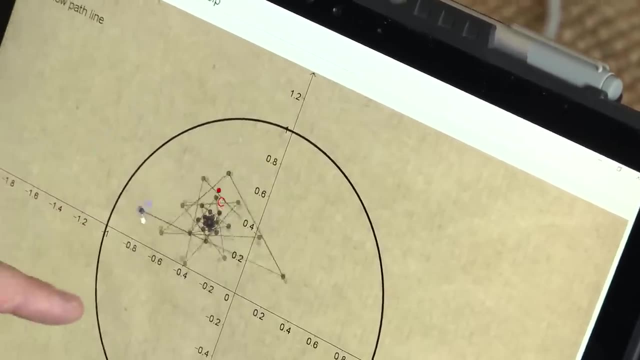 but somewhere else, outside the circle, unstable, And in fact it's not obvious where this is happening. Stable, unstable, stable, stable, unstable, no, stable, but over here, inside the circle, always stable, unless I go there. I keep saying the circle as if it's important, it's. 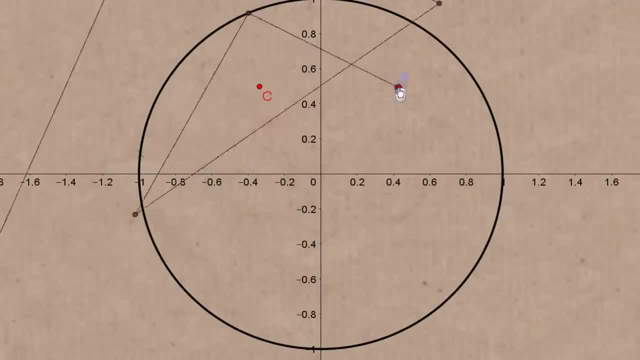 really not important anymore. The boundary is clearly not a circle, but it's kind of nice to move this around. I think that some places are unstable and some are stable. What I'd really like to see, and I hope you would too, is the boundary of stability, So let's see that, In fact. 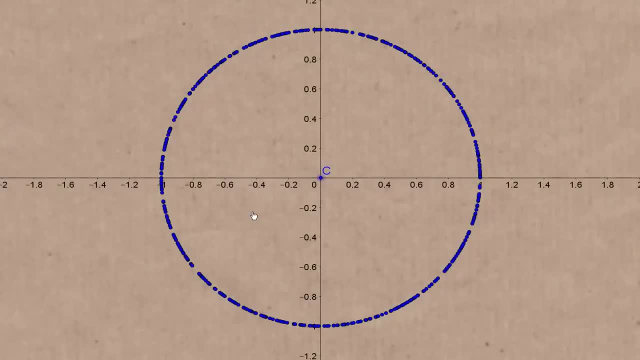 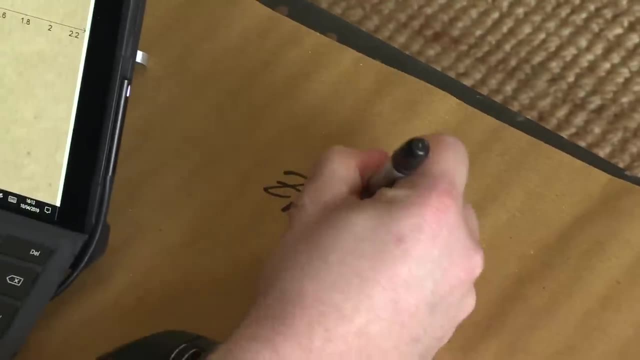 let's look at the boundary. If the number I choose to add each time is zero, you get the circle. That's like the simple iteration. If you choose to add something different, by the way, I'm going to write something down here. What I'm capturing is this iteration, which always looks a bit technical. 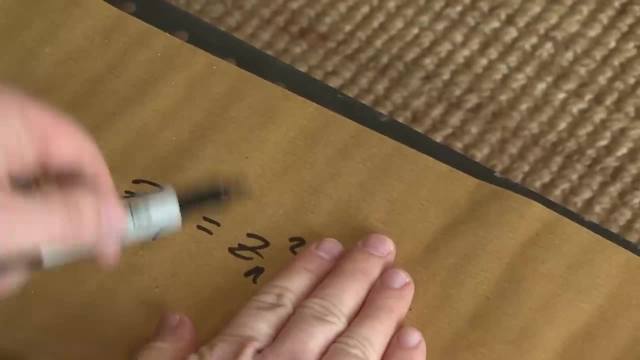 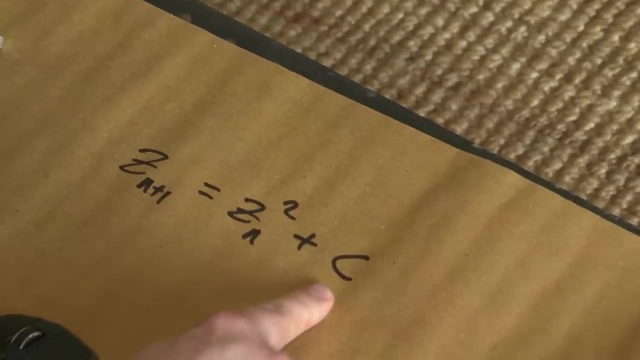 and if I cover that bit up, it's what we did at the beginning. I said: square a number and that's your new number: Square it, square it, square it. But instead of just squaring, you do square it, add something There, you see, for it's a constant, but it's a complex number. Now we're ready to look. 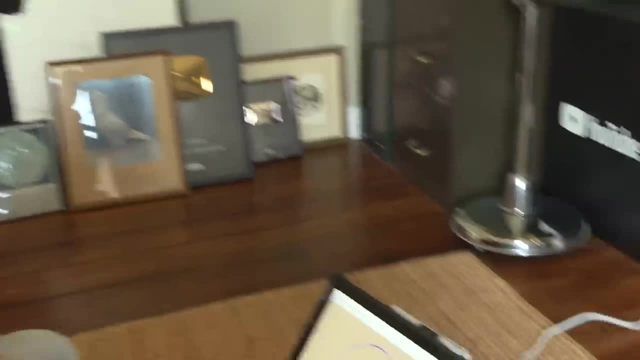 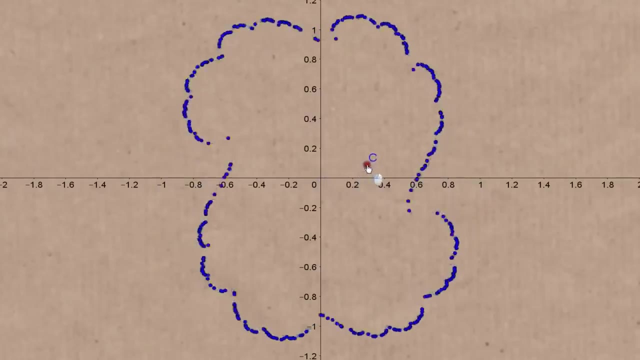 at that. If c is zero, you get a circle. If it's not zero, I see where my brain melts a little tiny bit. If c is not zero, the shapes become these shapes, And I always find this a little bit of a shock. There may be some familiar looking shapes, I don't know. 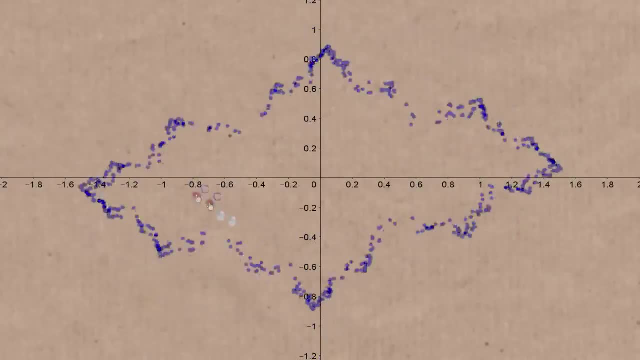 But sometimes they're not even connected together. They're like dusty little particles And these regions, particularly when there's obviously a region which is not a circle necessarily. they're called Julia sets And again Holly's done a really lovely video about Julia. 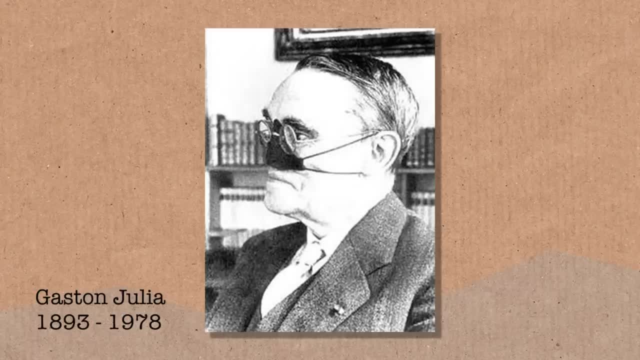 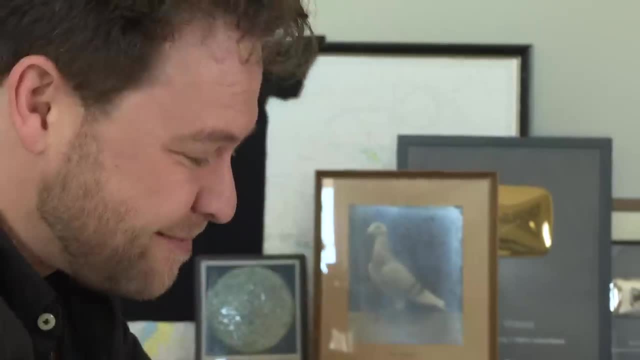 sets. There's a bit of history about Julia sets, found by Gaston Julia- hence the name- who was a guy, French mathematician, I think early 20th century. He did it without a computer. He wasn't able to just do this and move on, Jojoba, and see the boundary. He was doing this by hand and 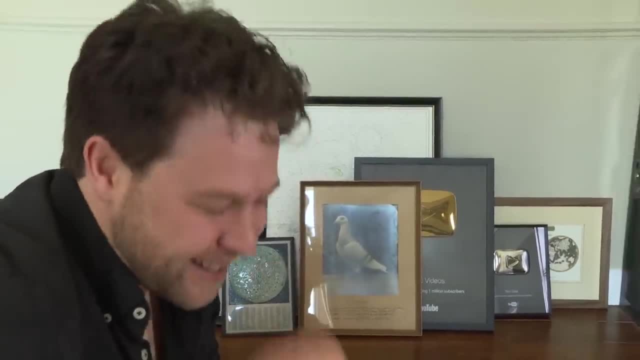 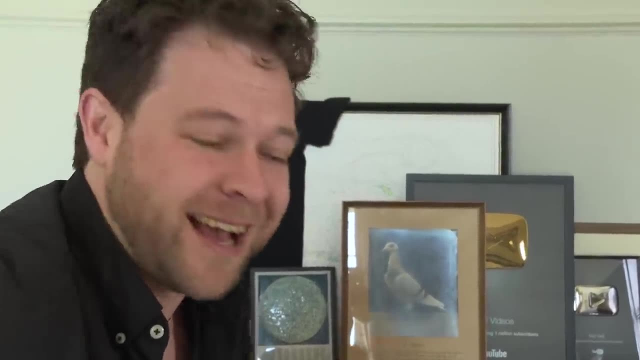 using some beautiful structure, Like I mean. every time I tell the story I'm like fair play. He also is really interesting in that he had no nose. Genuinely, if you go and find a picture of Gaston Julia, he has a leather thing across his face. His nose was damaged in, I think. 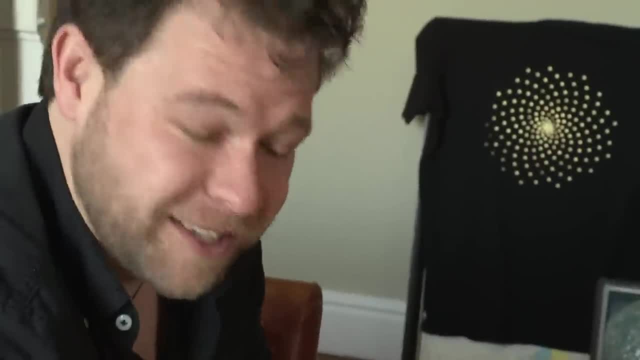 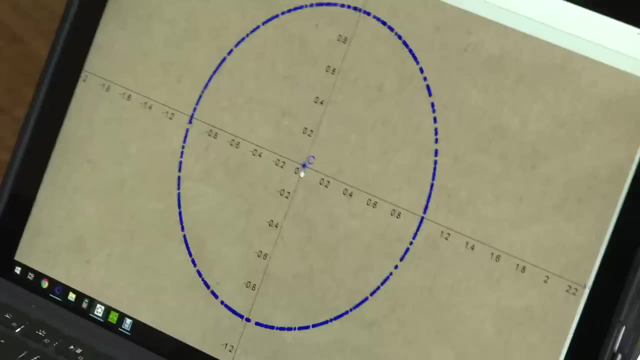 the First World War. Before I leave Julia entirely, the sets that you can see give you a little bit of a hint about what's coming. So let me show you two things about the Julia sets. First of all, the simplest one is a circle. It's not that exciting, But they are exciting but they're not. 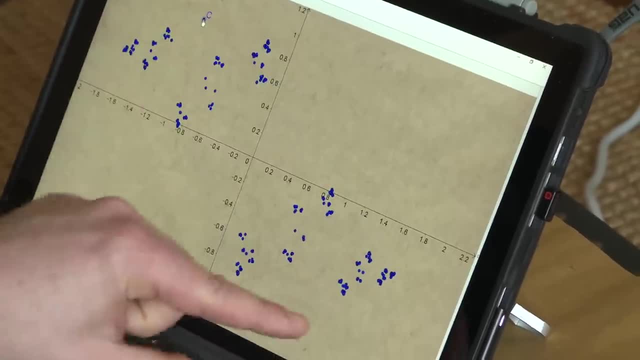 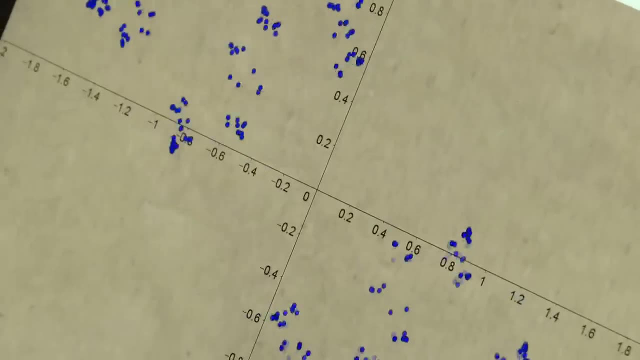 in this obvious region. Sometimes they look like they're separate regions. These don't look like they're connected. The way I'm animating it here they're all slightly dusty looking. That's just the way I'm making it happen quickly, But sometimes they're definitely not joined together. 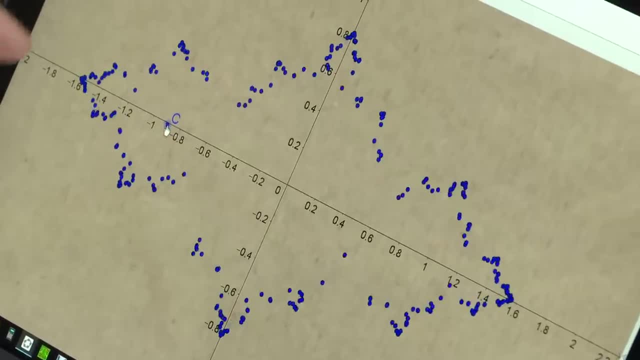 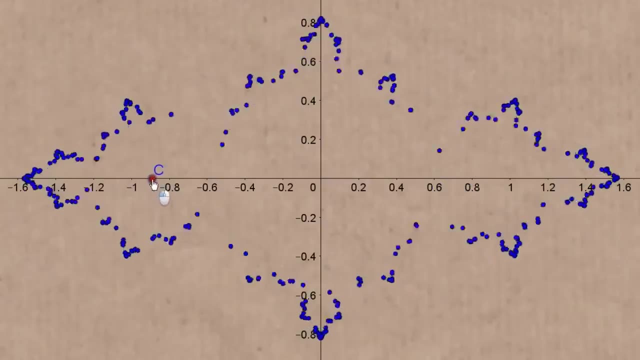 And sometimes they look like things you might recognize. The outline is looking vaguely like something I've hinted about this video may be looking like, But there is something important that Holly mentions in some of her videos about which ones are joined together, connected mathematically, and which ones are disconnected, separate like dust. Let me show you what they. 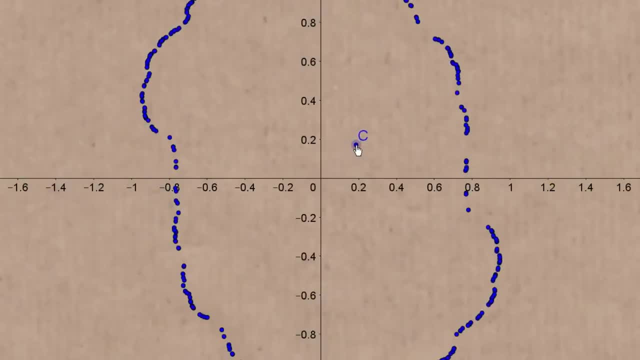 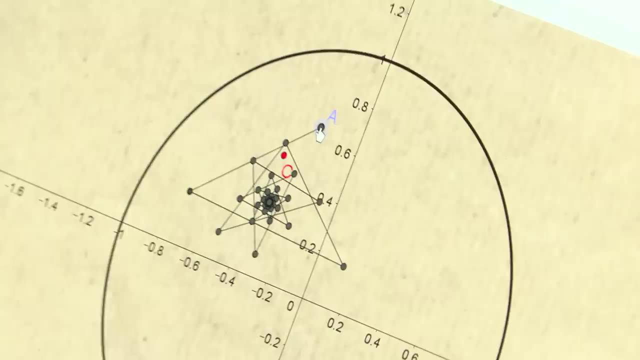 end up describing. So if we go back to this diagram, when I did the iteration, we were originally starting by you picking a number and squaring it. What happened in 1979 is a guy called Benoit. That was his first name. It didn't get better for him. His surname was: 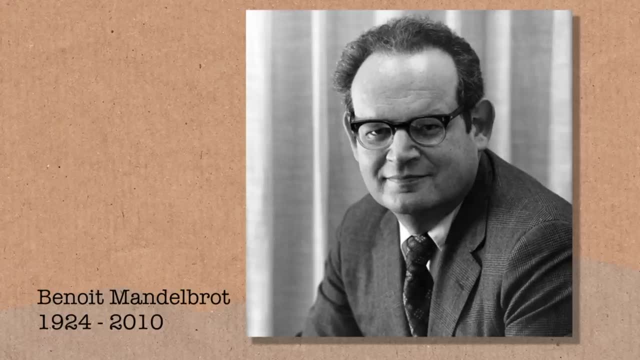 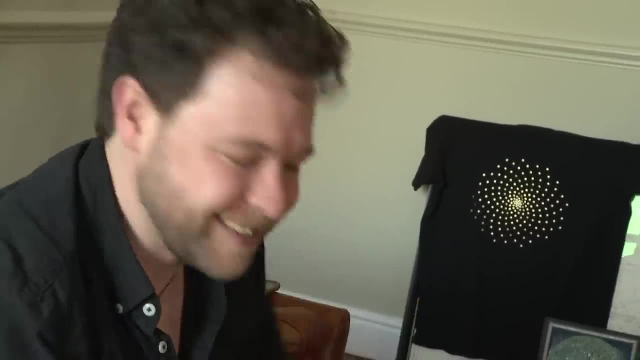 Mandelbrot. He's a very famous figure in mathematics these days, But it was 1979, 1980. It's kind of recent in the grand scale of mathematics. Benoit was like: hmm, I wonder what happens if I always start at zero, Instead of me saying pick a number. 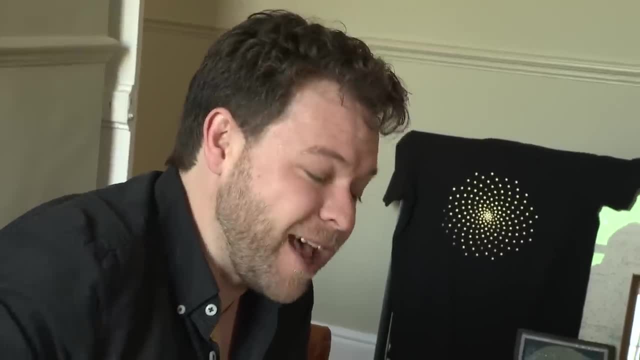 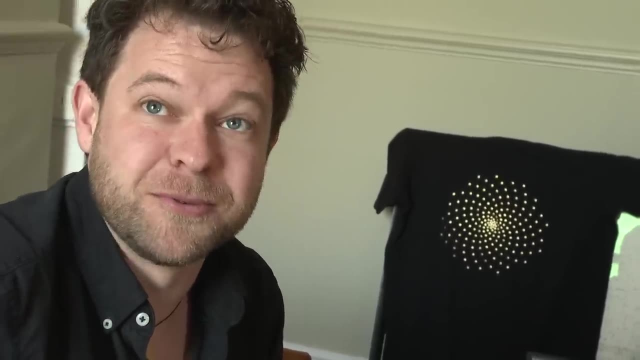 I would say like: pick a number as long as it's zero, And then all I really care about is what's the constant I add each time and which ones of those give me stable and which ones don't. Now, he didn't have a good computer. 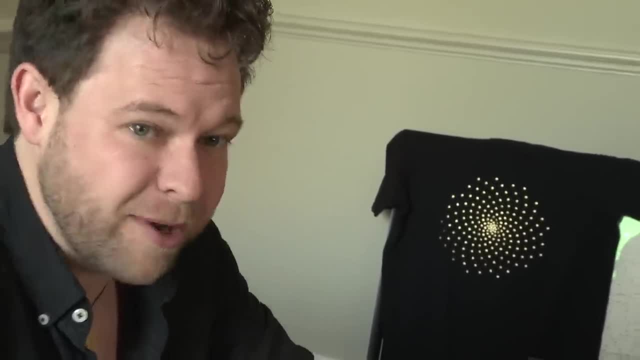 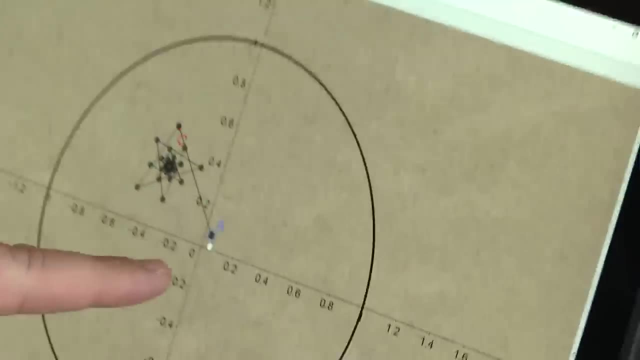 He was doing it on an IBM, working for IBM at the time and having to print out on a dot matrix or probably even pre-dot matrix printer. But we can kind of shortcut that, So let me show you what it looks like. Always start at zero and move the constant around each time. 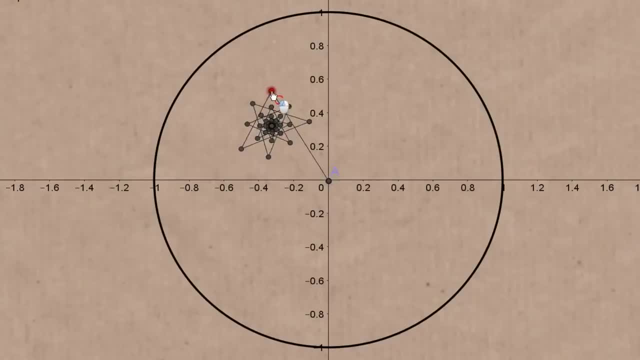 And if you do that, all you'll see is sometimes it's stable like this and sometimes it's different stable. I just really love this. I'm just going to move it around. They're kind of predictable and yet not predictable. You get spirally things. 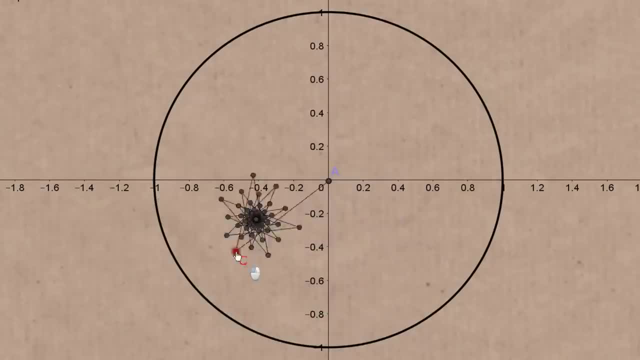 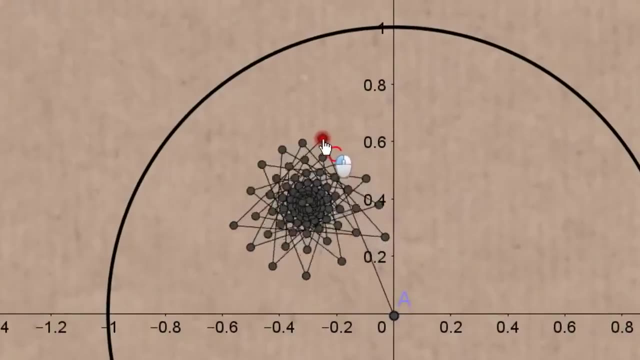 you get spider webby things and sometimes it's not stable, It's unstable. Sometimes it's got like: how many arms? is that Seven arms? Sometimes it's got three arms, Sometimes it's got something else And sometimes it's just rubbish. 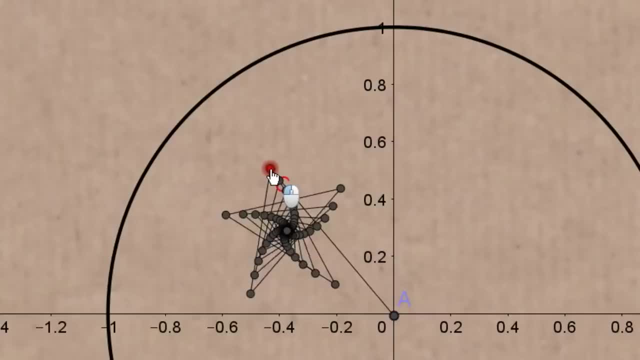 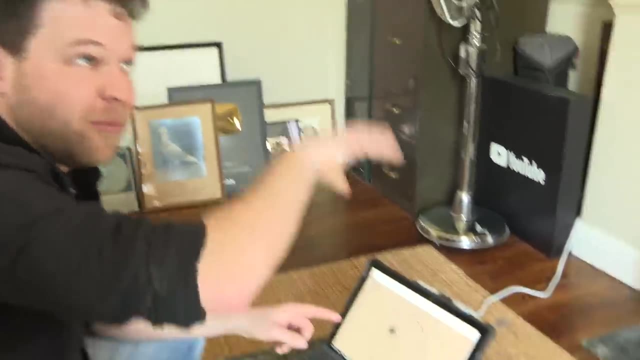 This is just the squaring, adding powering, Squaring and adding What they call. these are the orbits of. for every constant I pick which you mentioned, I picked one arbitrarily. it happened to be up in the top left there. This one, in fact, That's its orbit. 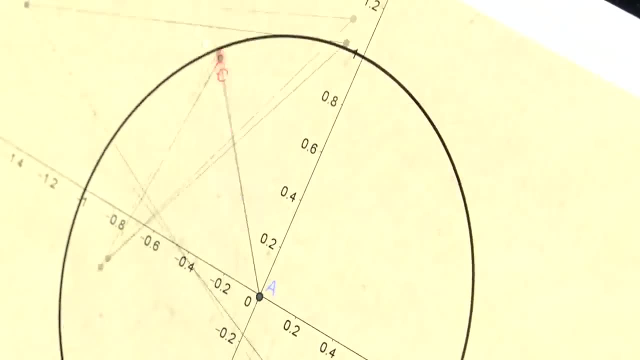 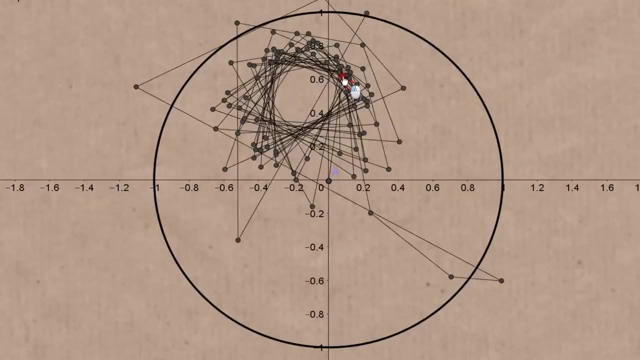 But any other constant you pick anywhere on the screen has an orbit, and some of them are boring, They're just gone And some of them are not. They're stable And some of them are not quite sure what the hell's going on. Excuse my English there: The idea that 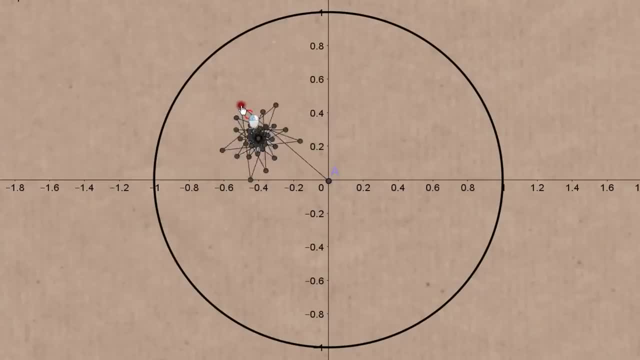 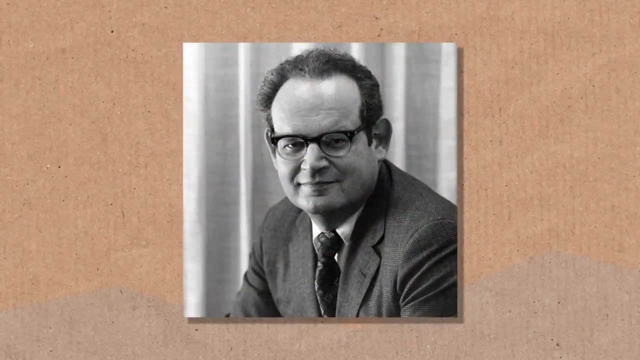 maybe some points are special and some are not- is what Benoit Mandelbrot first began to investigate. Other people were investigating it, but it ended up with this idea getting his name on it. So let me simulate what he first saw. Remember, he didn't have a monitor on his 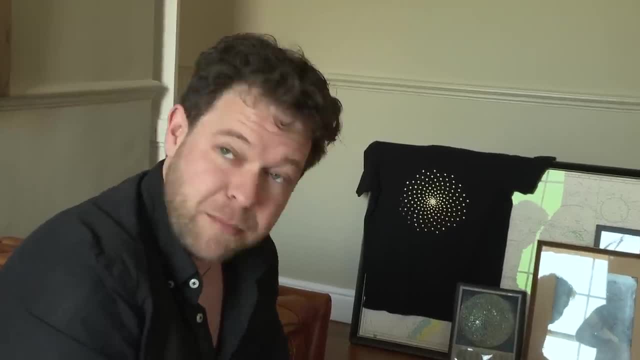 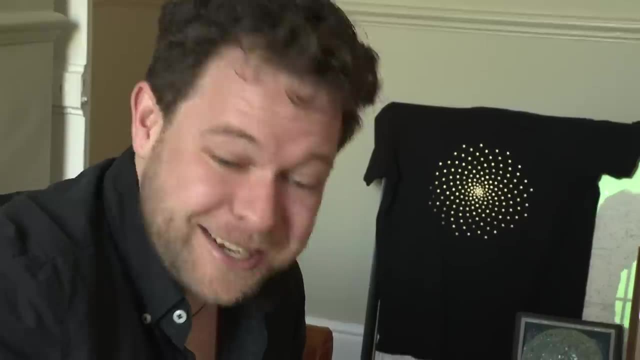 computer. He had a printer. He typed some code in: If you want a picture, you print it like 10 minutes later, after you've solved all the printer problems which still occur- Weird. He then has got to go and look at what he's like. have I broken the printer or have I messed my code up? 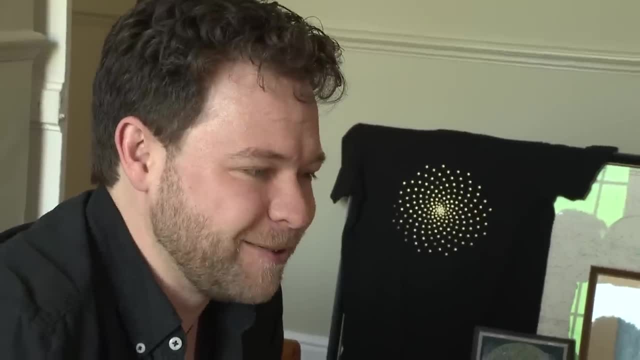 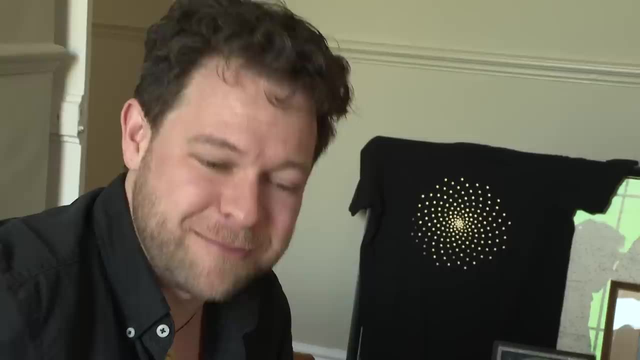 or is what I'm seeing actually real? And what he found was that what he saw. the technicians got there first and they were like, well, he's got it wrong again, And they cleaned up his images and took all the sort of dust that they assumed were printer artifacts. They're like 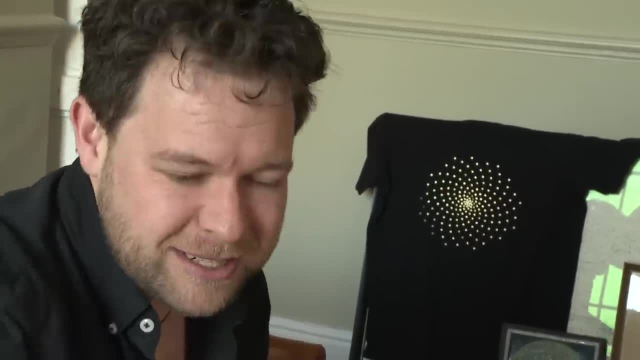 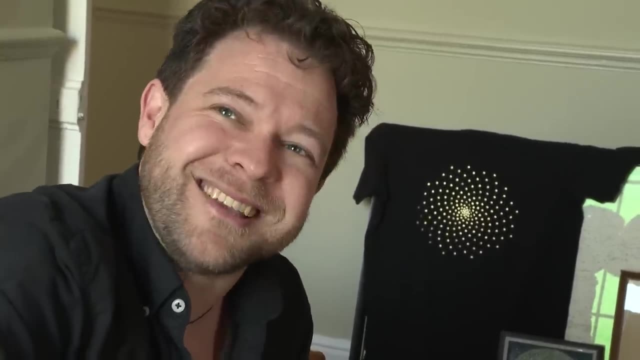 there's this smudgy bit here, Clearly not meant to be there. We'll just like: chop that off or tell the printer. And he eventually had to go to the technician and say, like my prints keep coming back different from what I expected. They're like: well, we're just cleaning them up. He's like: 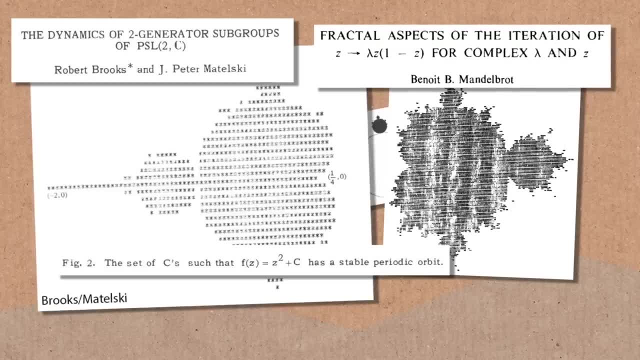 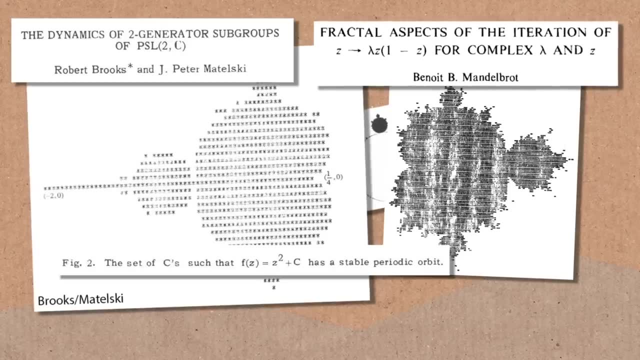 stop cleaning them. I think what I'm trying to see is a weird messy, dusty looking thing And they're like: oh, you want that. I don't know exactly what happened. There's a really good book by James Glick called Chaos which kind of tells that story worth a read, but I'm going to 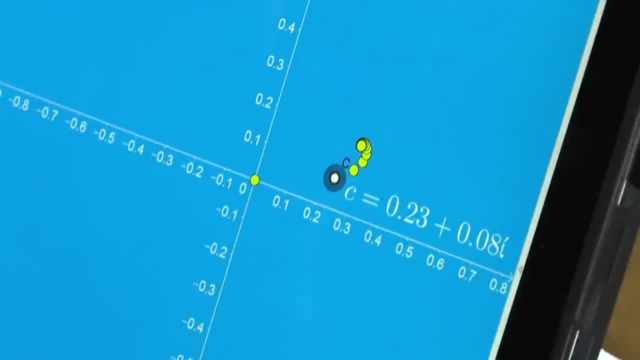 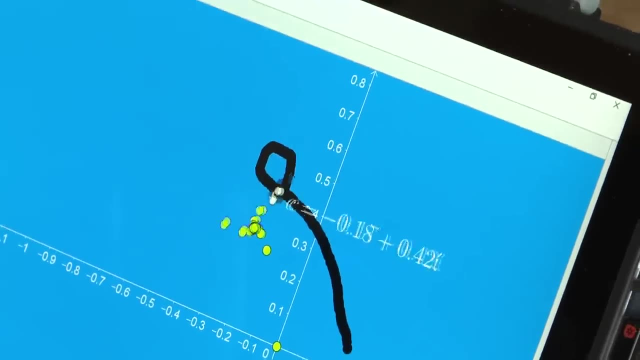 simulate the dust that he saw. I'm sorry about the lack of brown paper, but there's a reason for the color. This is the same orbit thing I was showing you just now. Can you see? there's like a spirally three there, but I'm leaving a black trail because I'm telling George to colour the screen. 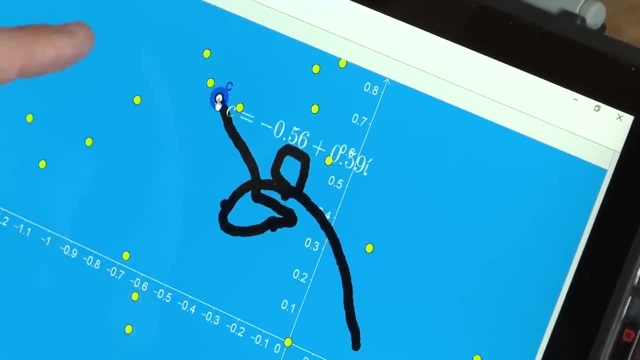 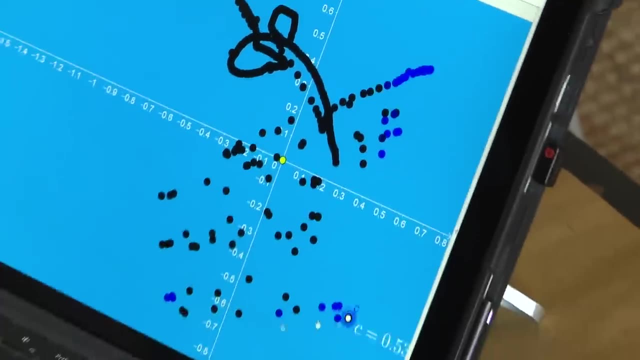 black if it's stable, and if it's unstable, like that one, it goes blue Black, blue, stable, unstable. And I'm on the screen Now. this is not going to make a good picture, but I want you kind of to feel. 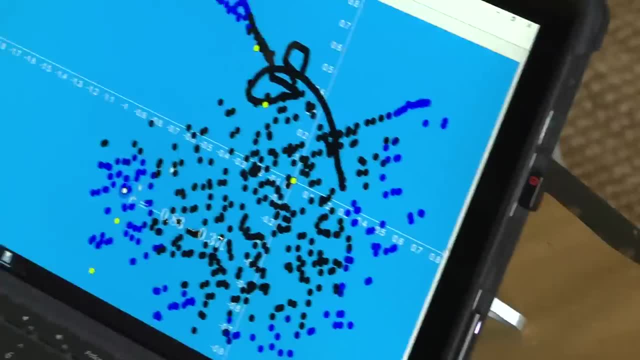 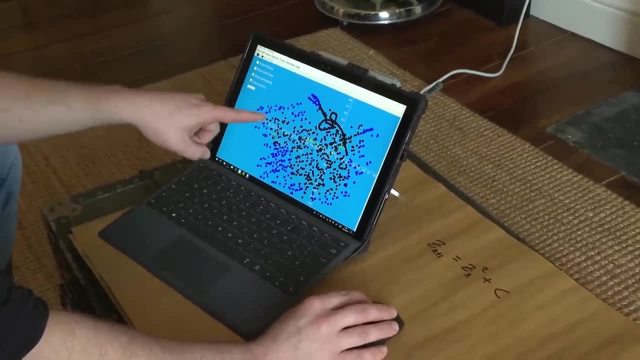 what Mandelbrot felt like. So he was seeing black and blue dots, or in this case, probably just white and black dots- Black for stable and, in my case, blue for unstable- And he started to wonder why there's a black region here that's not over there, It's not symmetrical. I really think it must have. 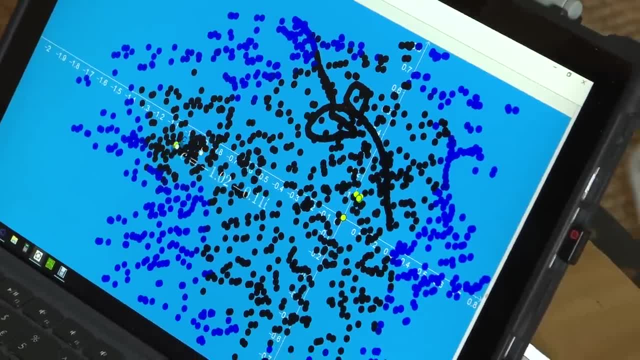 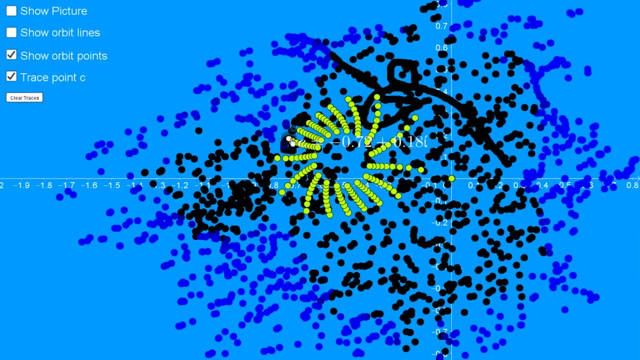 felt something like this when you have a rubbish printer and you don't trust your code and you wonder what the hell are you seeing? So this is going to take ages. right, I'm going to shortcut the process. What he eventually saw, in higher resolution than he saw, is this picture: 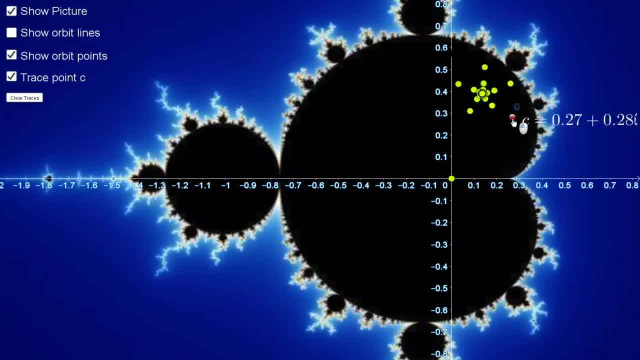 And the black regions, like I was colouring earlier, are stable. You can see anywhere I go in the black region you get a nice stable pattern with lovely orbits, and that's the thing I love seeing move. But if I go over the edge, unstable, Stable, unstable, stable, unstable. So it's. 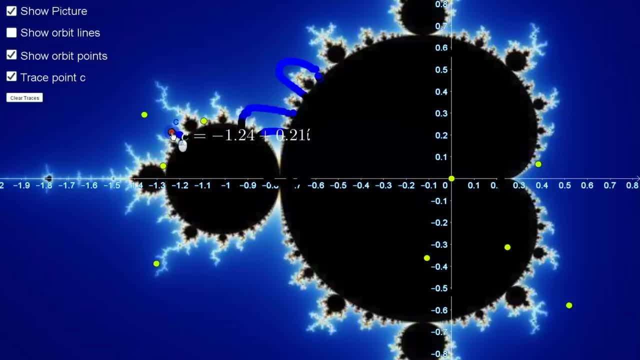 even stable in this region. It goes into like two piles. but if I go outside the region disappeared. If I go up here you get into three piles And in fact Holly's done a lovely video on how many piles you start making depending on which of these little bulbs you go into, But the first. 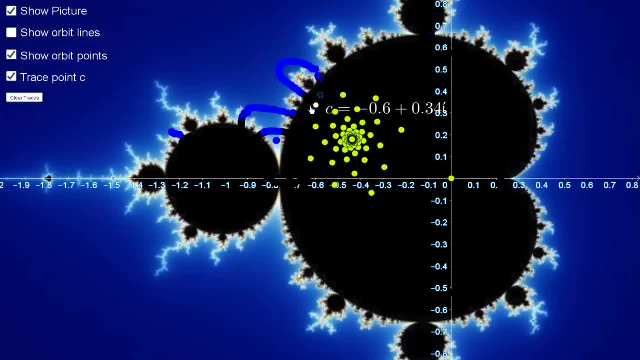 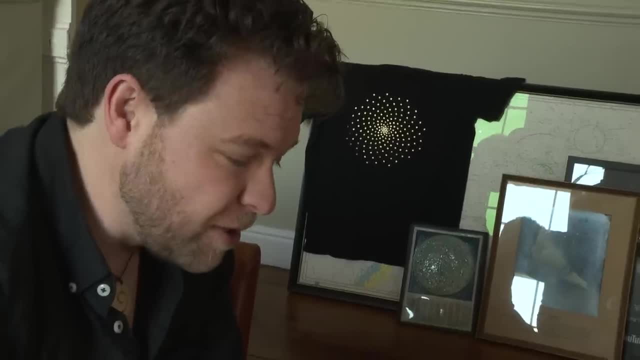 time that Mandelbrot saw this, he had no idea about any of that structure. He just saw a shape which shocked him. First of all. it's beautiful. It's kind of weird, But getting a viewer to display it like I've got on the screen. now you can go and watch any number of YouTube. 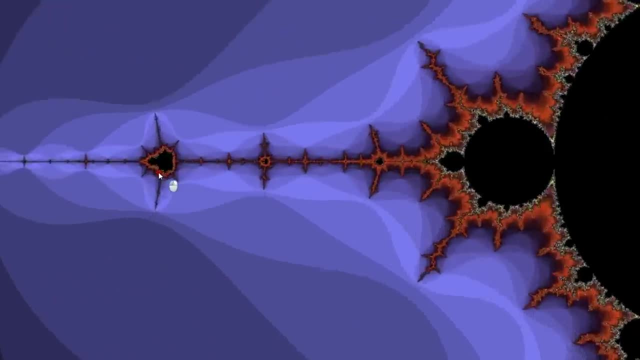 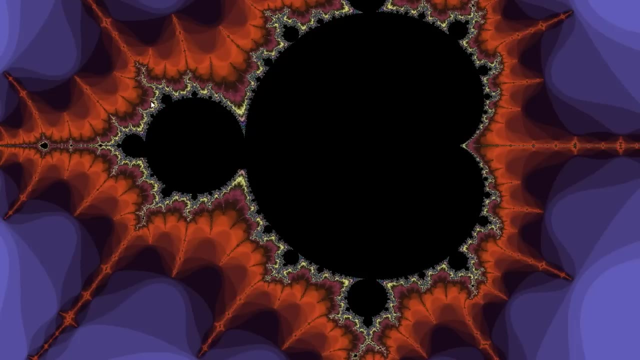 videos and zoom in on it. But you can see what Mandelbrot couldn't see, that he saw this little blob and thought I wonder what that is. And he had no idea until he wrote his code better that it was another version, not quite the same, And you can just zoom in forever And now. 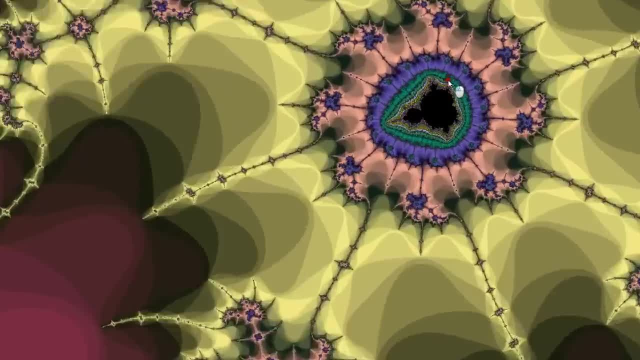 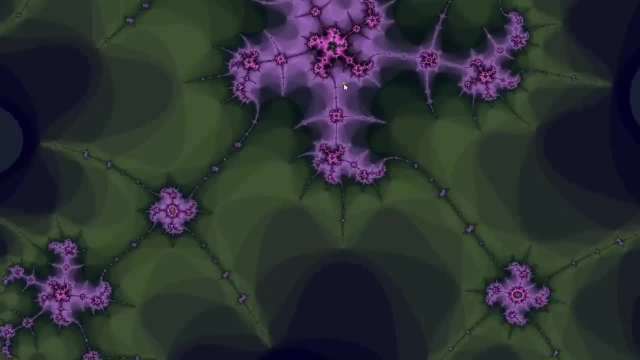 I don't think YouTube needs more videos of me zooming in on the Mandelbrot set. However, I'm going to do it anyway. Ben, why are there different colours, Like it's not always black and blue? Absolutely So. the original Mandelbrot set that Mandelbrot saw. 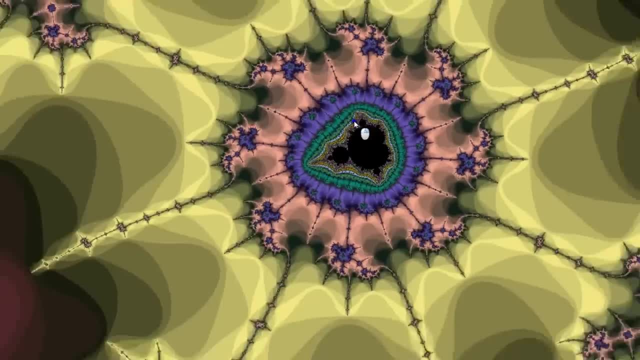 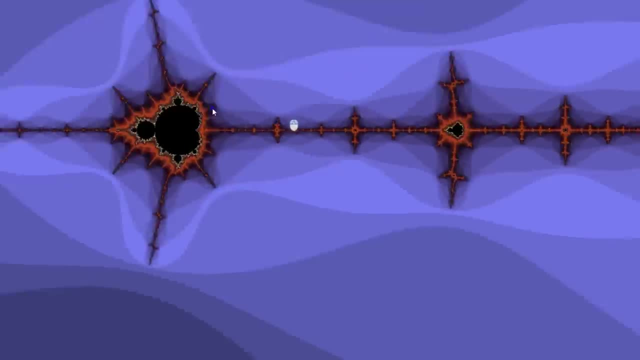 was two colours: Stable, unstable. black, white or whatever I did, black and blue. The colours you're seeing in this are an arbitrary decision, but they're not as arbitrary as you might think. So let's go back to the original, which is out here. Black for stable, but the colours indicate that it's. 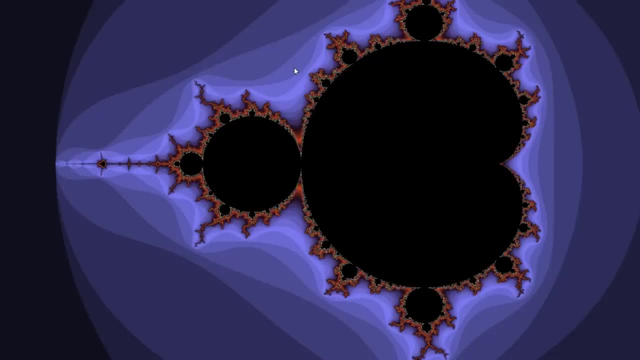 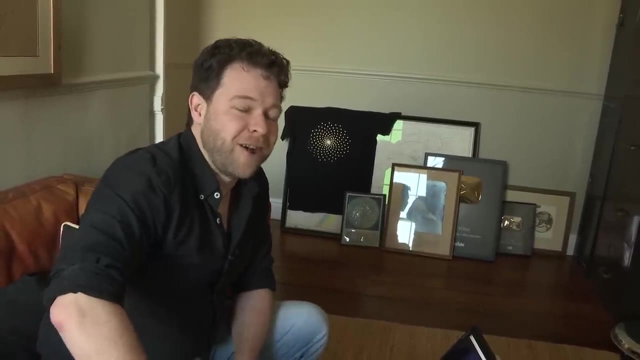 unstable, but the colour indicates how unstable. And so, if you think back to the very first question I asked you, I said: square it, square it, square it. And within two iterations you're like: no, because it's big, And that's an indication that you don't need to ask any. more iterations to know what it's going to do. With complex numbers it's less obvious what it's going to do. It's much harder to predict. but eventually we proved mathematicians- I say we, not me- mathematicians proved that if you go outside a circle radius two, it's never coming. 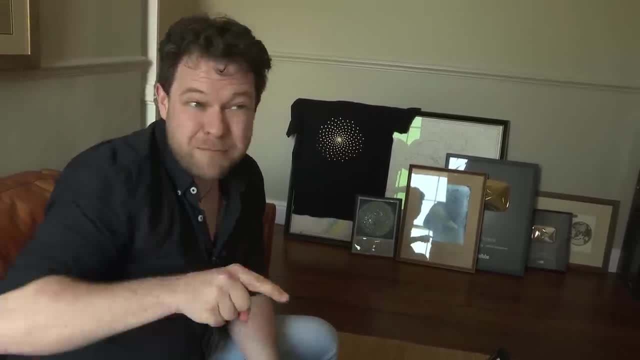 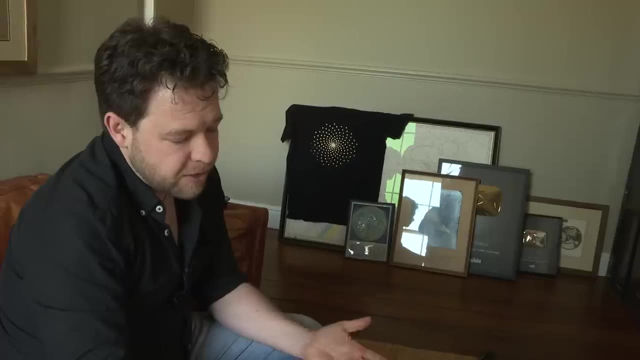 back. But if you're inside, you can't guarantee it. It might be bouncing around near the edge and it might stabilise again. And you see, some of the orbits are complicated. So all you do with the computer is you ask it to check, let's say, 200 times. 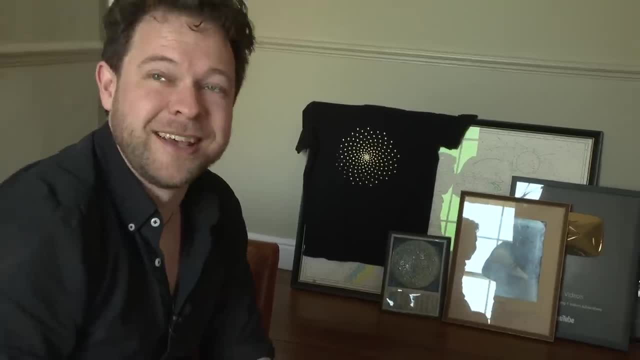 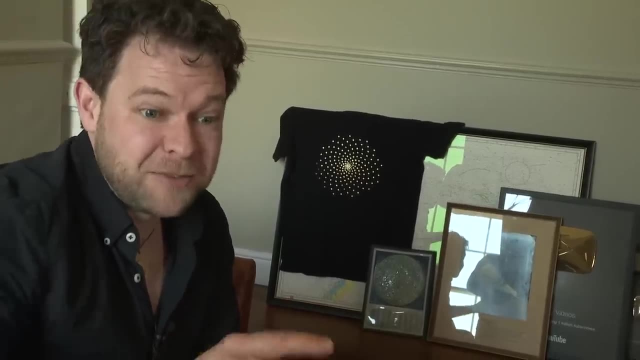 And if you're still inside radius two circle of 200, you're like, let's colour it black, It's probably stable. But after like 50 iterations, if you've just crossed outside, you're like, well, now I know it's gone, But maybe the next time you check it takes 60 iterations. 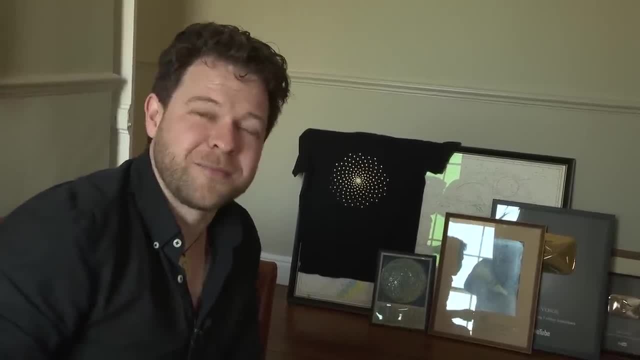 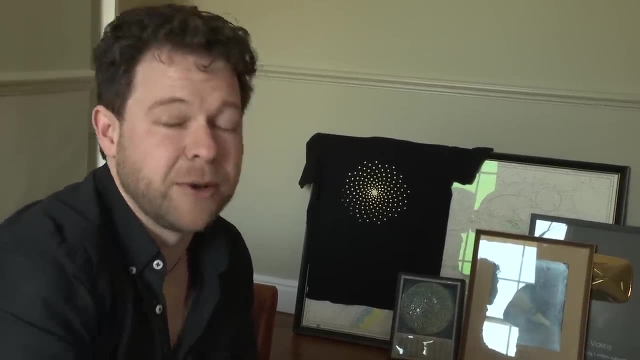 And you're like: well, that's less unstable. Maybe I could colour that differently. That was a long way of saying the different colours on the image are the different levels of instability. Really, it's how many times you checked before you knew they were going to explode. 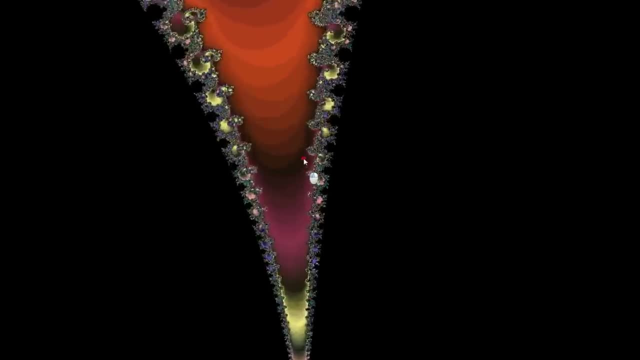 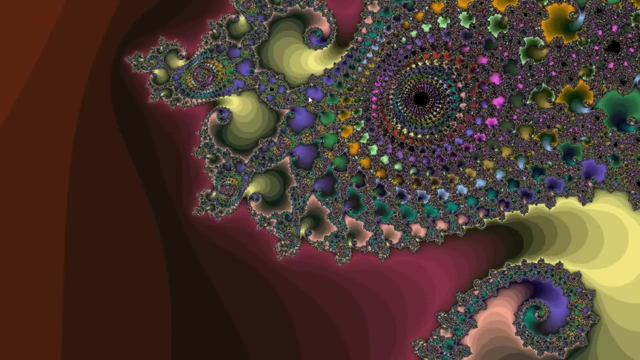 And what matters when you zoom in is that the colours change really, really quickly. So all the colours on the screen here are indicating that a tiny movement of the original point gives you massively different behaviour, And that's become what we call the sort of hallmark of chaos theory. now is where 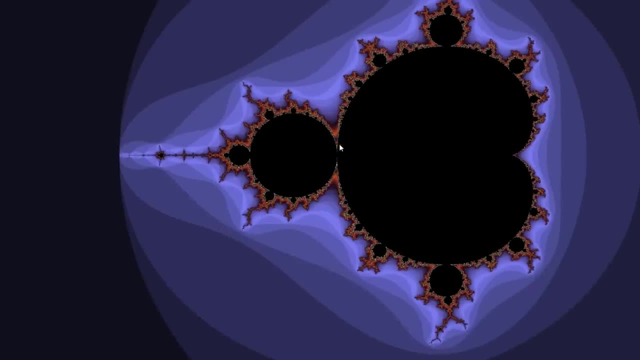 a tiny change gives you fundamentally different behaviour. On the Mandelbrot set, you move your chain. every point you make is dependent on which C you pick. But Julia set you fix one And I can turn this software into Julia set mode. I'll do it slightly first. 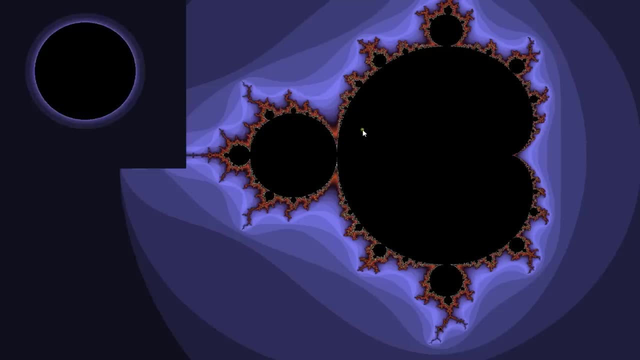 press J on here There's the circle which is the original Julia set And that's in the middle here. But if I move the mouse around you see the Julia sets with different values of C start changing beautifully. Like it's just a quick sketchy animation, but it's already much. 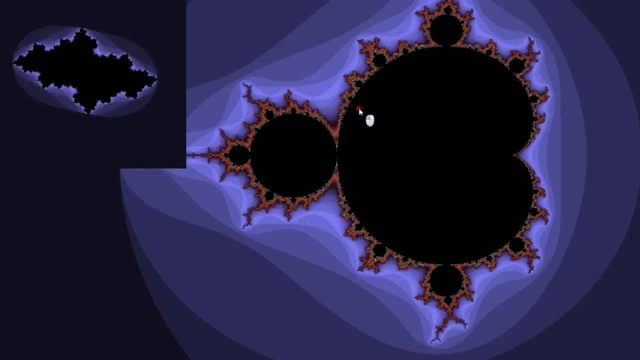 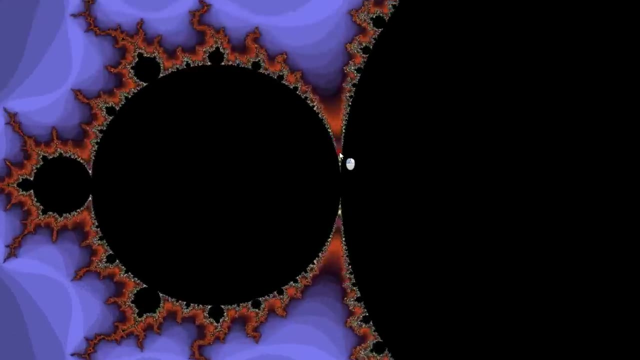 more nice than the outlines you saw earlier. And what I love about this is the Mandelbrot set is kind of like a map of Julia sets. So if you go and find a bit of the Mandelbrot set down here, this is called Seahorse Valley because it kind of looks like you've got loads of seahorses spiralling around.